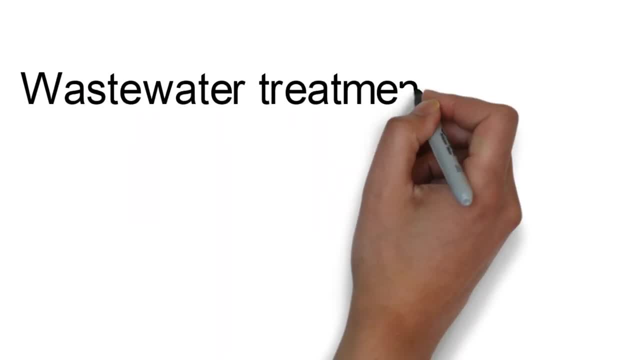 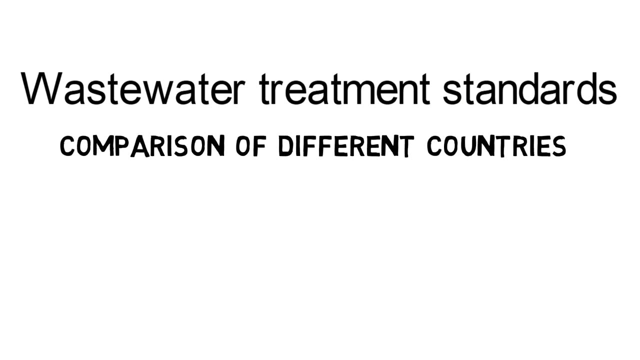 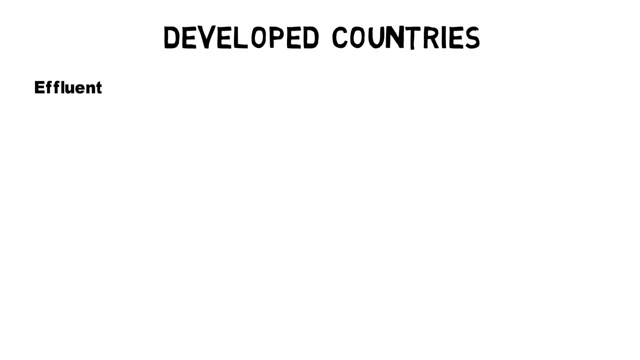 In most developed countries, standards for wastewater treatment are continuously improving. Compared to the 1970s, the effluent requirements for the most important pollutant indicators – BOD, CO2, nitrates and phosphorus – have steadily increased, For example in the United States. 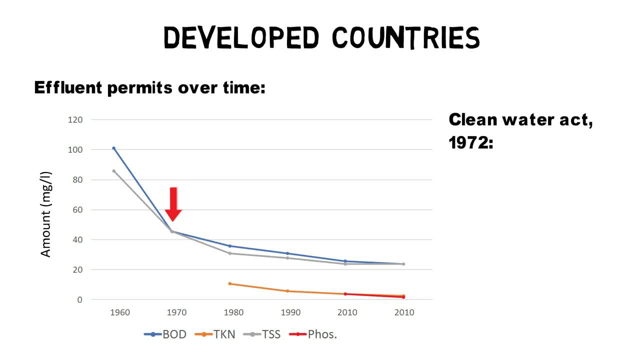 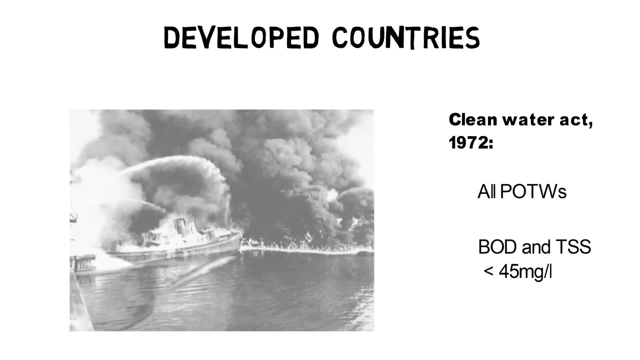 the Clean Water Act from 1972 demands that all municipal sewage treatment plants are required to meet a weekly average BOD and TSS effluent value of 45 mg per liter or less. Before 1972, two-thirds of all wastewater was let untreated into natural waterways. 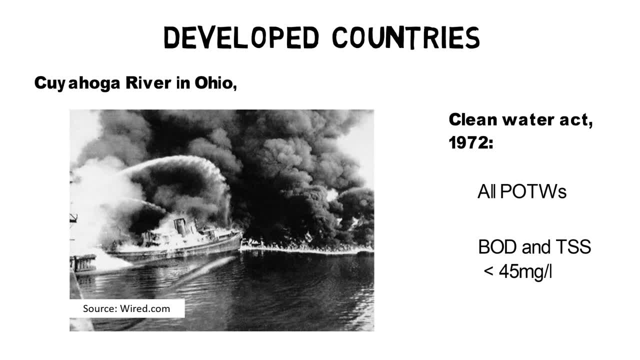 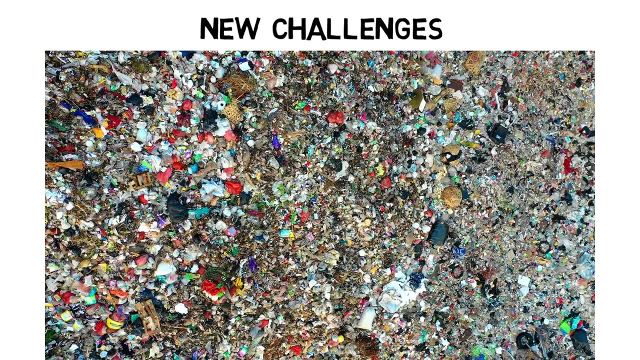 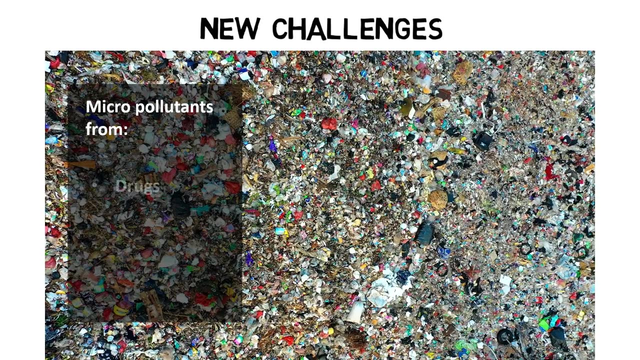 causing that. some rivers, like the Cuyahoga River in Ohio, were so foul that they caught on fire. Nowadays, the occurrence of micropollutants creates a new challenge for wastewater treatment in developed countries. Micropollutants originate from drugs, personal care products, pesticides. 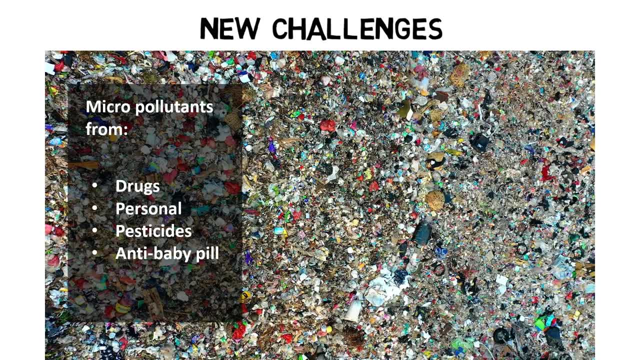 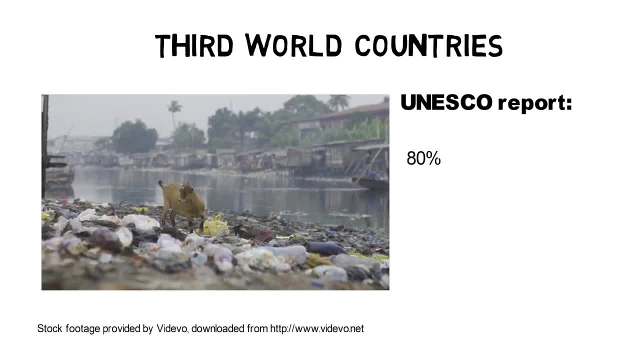 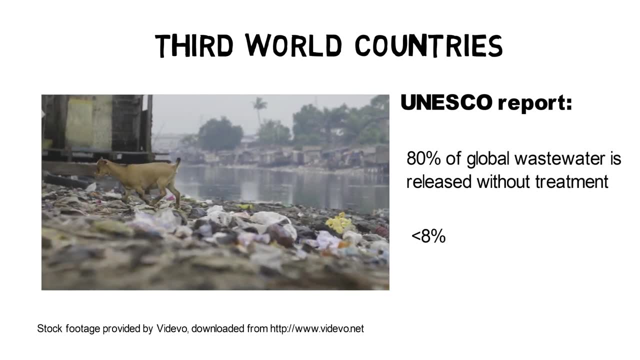 and the anti-baby pill and enrich more and more in rivers and lakes. The UNESCO estimates that worldwide over 80% of wastewater treatment in the United States is released to the environment without adequate treatment, Especially in third-world countries. less than 8% of all wastewater is treated before. 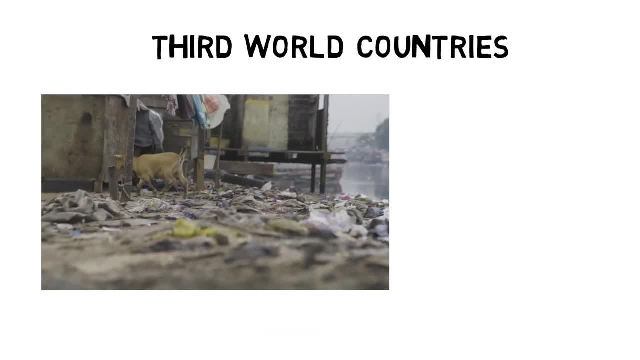 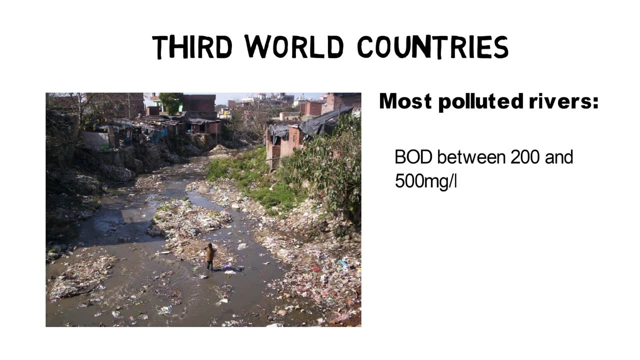 it is released into natural waterways. Some of the most polluted rivers in India show BOD levels between 200 and 500 mg per liter, such as the Markanda River in northern India. As mentioned earlier, since the 1970s, the minimum requirement in developed countries 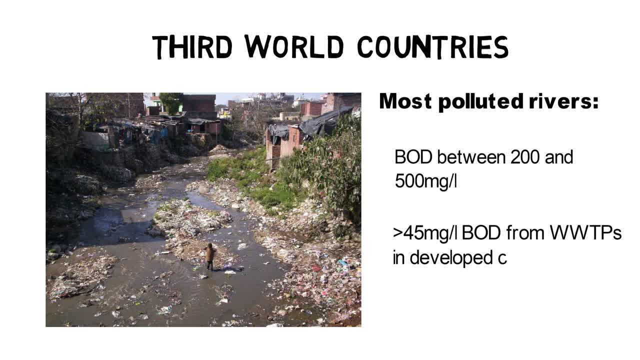 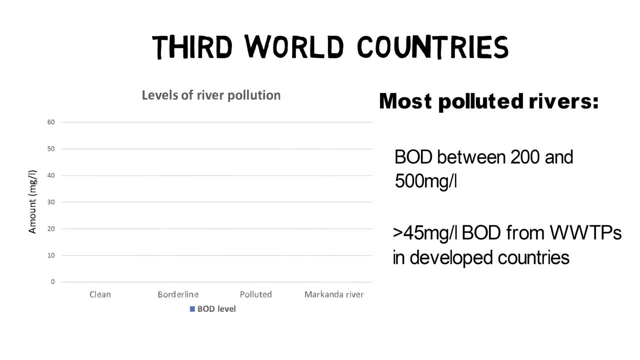 for BOD from municipal wastewater treatment plants is 45 mg per liter or less. When treated wastewater is released into natural waterways, it is further diluted so that rivers with a BOD below 8 mg per liter are classified as clean. below 20 mg per liter classified. 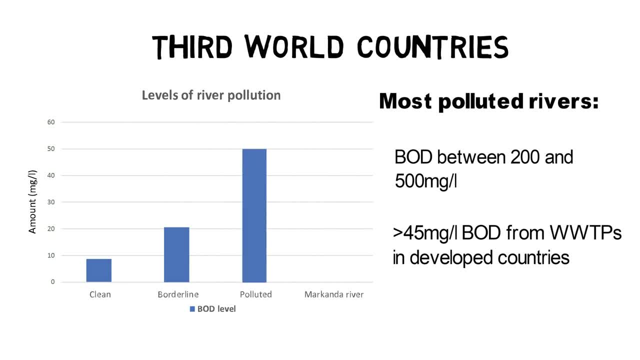 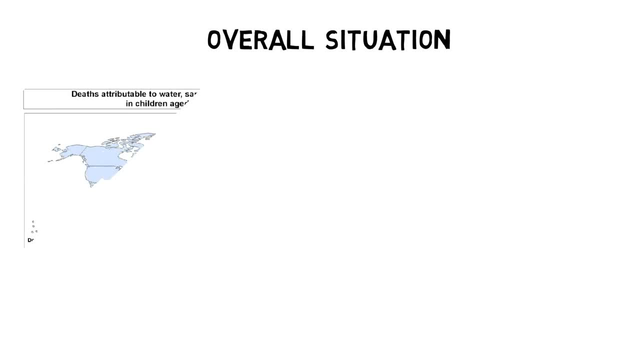 as borderline water and rivers with a BOD above 20 mg per liter are classified as polluted. Consequently, several waterways in the United States, including the Cuyahoga River and the Guadalcanal River, are regulated by the UNESCO.